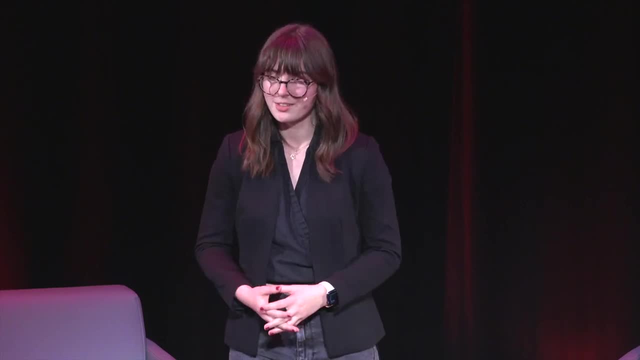 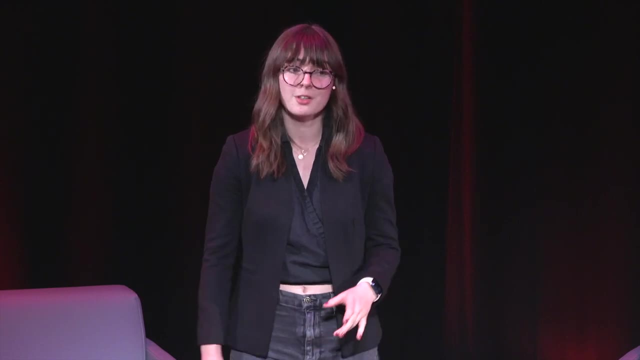 was beyond excited at the chance to learn some new engineering. I was excited to learn some engineering skills. What met me was not what I expected. Instead of a fun educational culture, I floundered and developed a serious imposter syndrome. The upperclassmen I met were condescending. 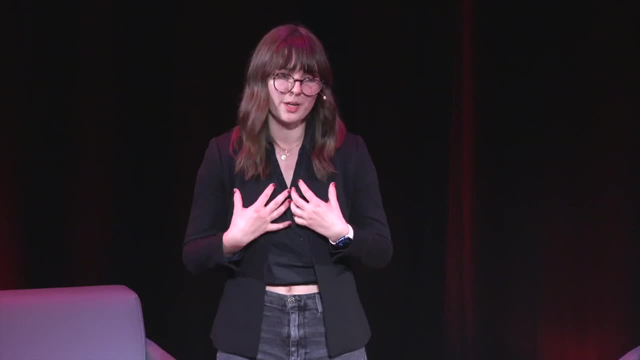 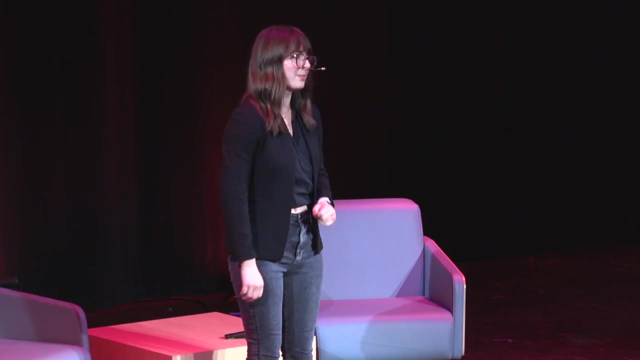 and preached innate engineering talent, which convinced me I wasn't good enough or smart enough or engineering enough to meaningfully contribute. In those short months, my life plans and dreams did a complete 180, and I turned away from engineering and robotics and turned towards finding a new passion, one that I felt I could meaningfully pursue. 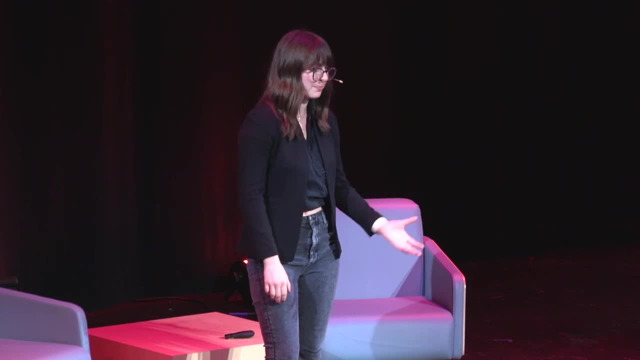 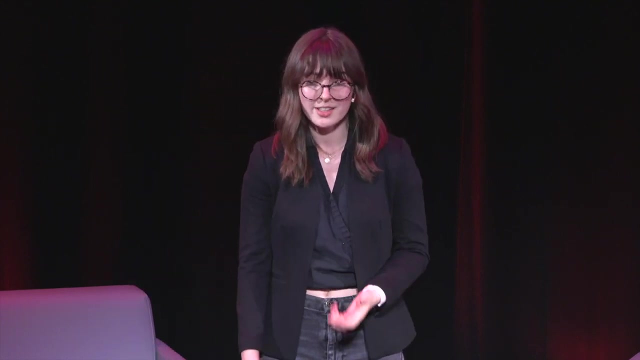 Then, in 10th grade, we still couldn't return to the lab because of COVID, and we didn't build a full-scale robot. So I turned towards physics as my passion of choice, convincing myself it was something I loved. Finally, in 11th grade, we returned to the lab. However, all of the condescending 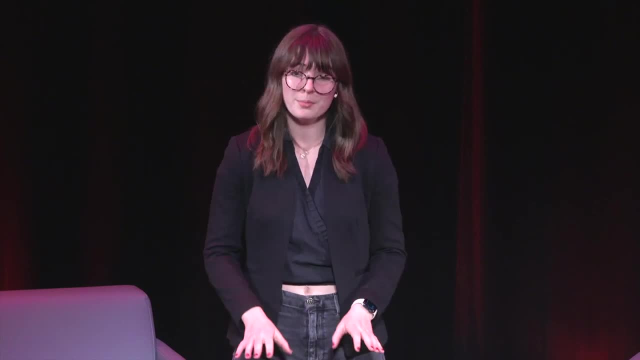 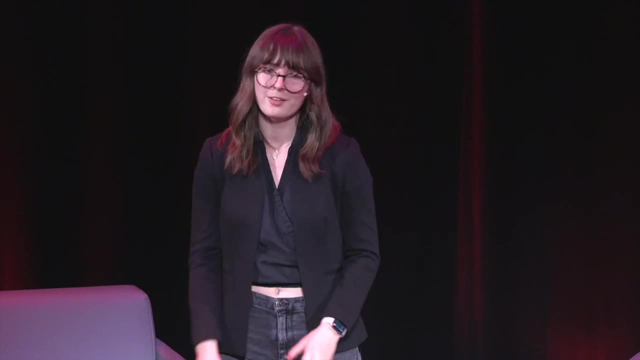 innately gifted upperclassmen from before were gone, leaving behind a team that knew next to nothing And, crucially, carried over little from the previous generations. No more condescension, no more superiority complex. Instead a chance to build a more inclusive team culture. 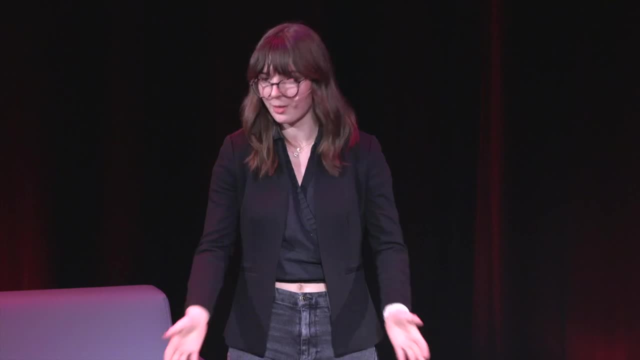 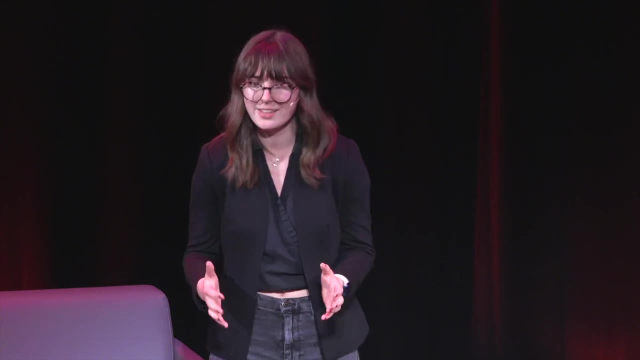 That was the year that I was offered a leadership position on the team and, although I was still living under the weight of the former leader's words, I was determined to create a cultural shift on the team towards a strong, safe and supportive environment. 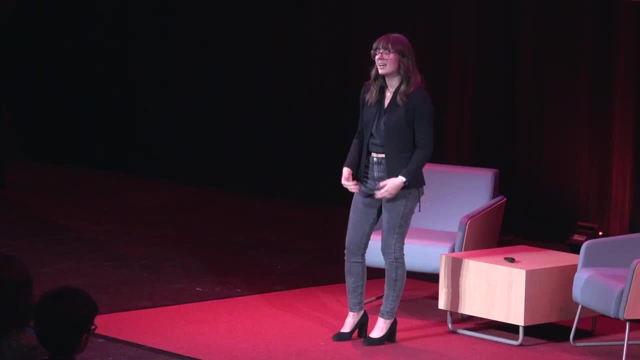 This is my story. It has shaped the way I interact and communicate and the way that I approach robotics. When I think about solving the issue of sexism in the STEM world, I reflect back on my own stories and the experiences I've heard from others, And these stories and experiences shape my 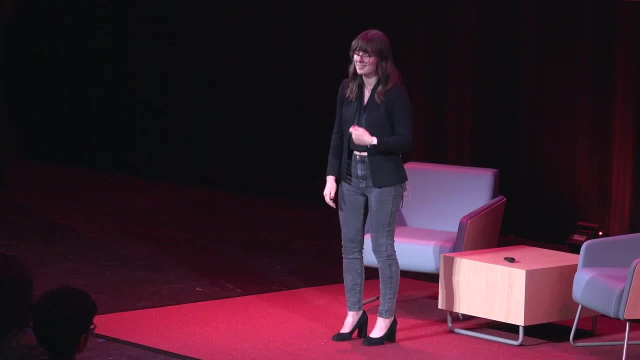 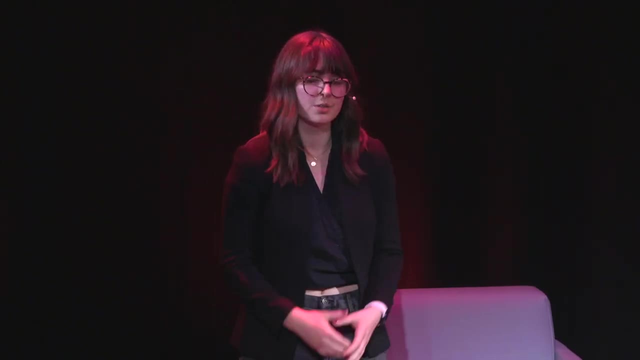 response to the issue, showing just how important the ask step of the process is. The second step in the process is research. Engineers do research to examine the engineering, the design problem in more depth and to learn more about these current solutions out there. 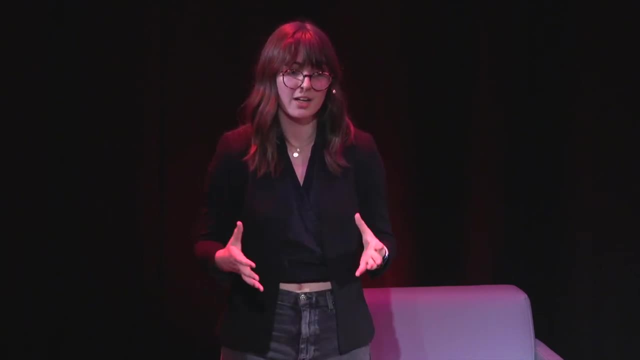 We can do research the same way to learn about the greater context of the issue we're trying to solve. Let's dive into some of the stats surrounding gender diversity in the STEM field. Although the wage gap is remarkably small for engineers, in other STEM careers only about four sense different. 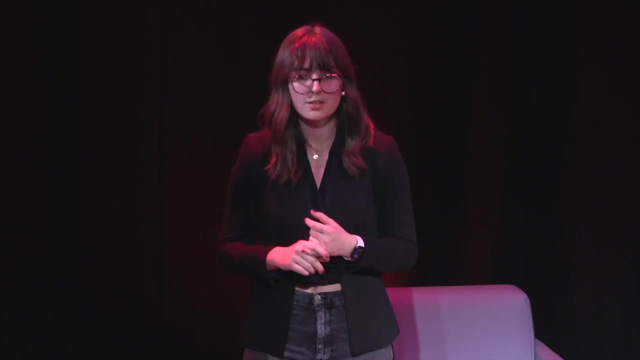 for robotics engineering, which encapsulates primarily mechanical software and electrical engineering. The only about 7% of robotics engineers are women, and that number can be as low- it is 1%- for more clean and no really reputable areas than not of a maintenance field. robots engineers are women, and that number can be as low as 1%. for more mechanical software and electrical engineering, Robotics engineers acquire women and accrue less. váse is and thus amplifies the ability to do research without being unclassified in the background. 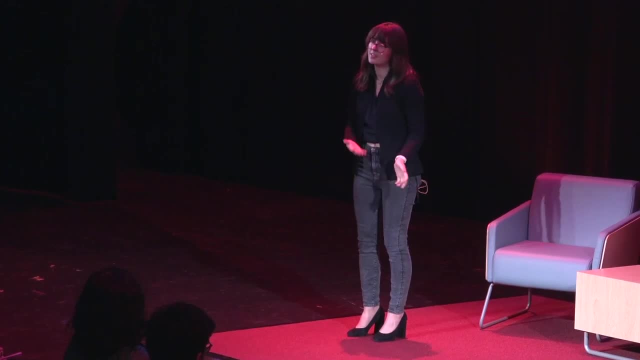 can be as low as 1% for more specialized jobs, such as senior electrical engineer. This is according to Zipia. Additionally, according to the Pew Research Center, women in STEM careers are more likely than women in other careers to indicate that they have faced gender. 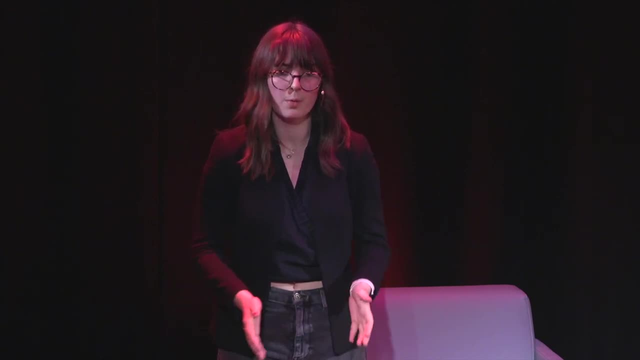 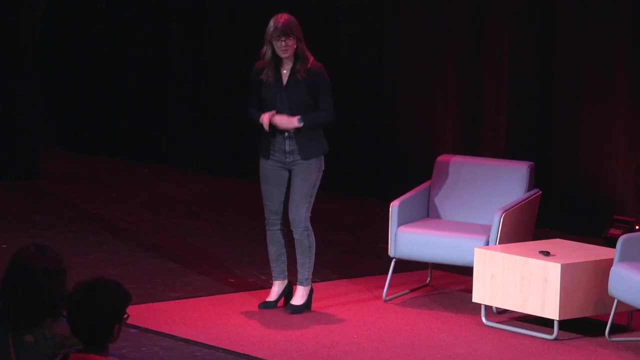 discrimination in the workplace. That's about 50% to 41%. All of these stats show that sexism isn't an issue isolated to robotics teams or even high school in general. Instead, Richard's highlights just how widespread the issue is. The third step in the process is imagine. 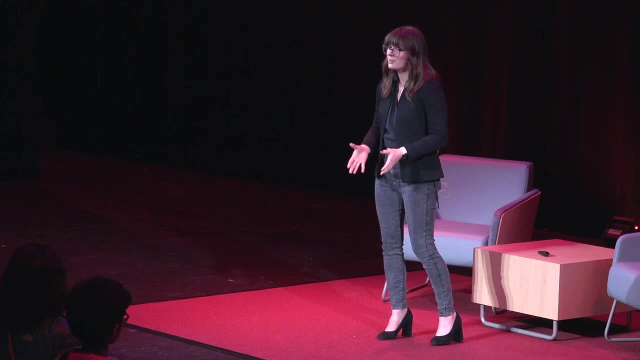 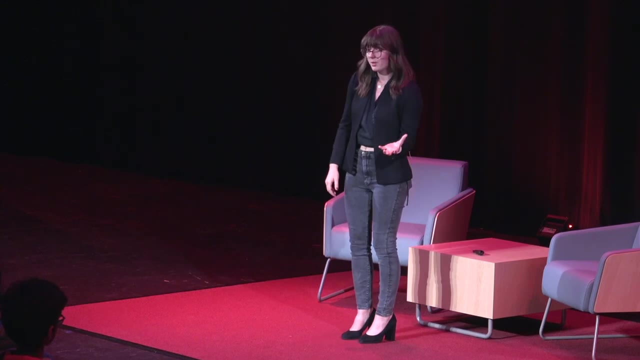 Now engineers use this step to brainstorm all of the different solutions to a given problem, but I'd urge us to take that a little bit farther. Now that we have a perspective on the issue and some research surrounding it, empathy must come next in our understanding. 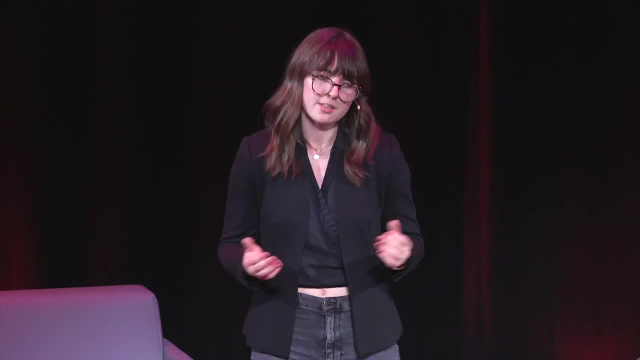 of the issue itself. Empathy goes beyond a simple understanding, but involves really imagining what it would be like to be able to do something about it. Empathy goes beyond a simple understanding, but involves really imagining what it would be like to be able. 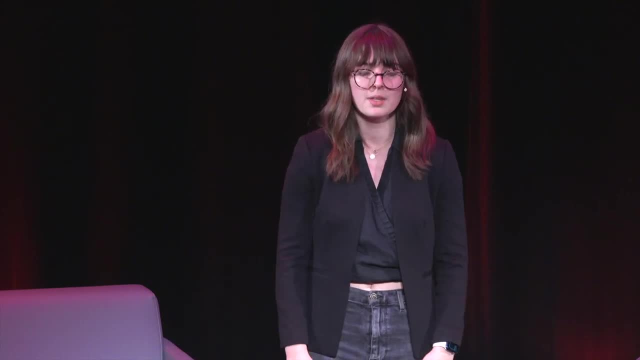 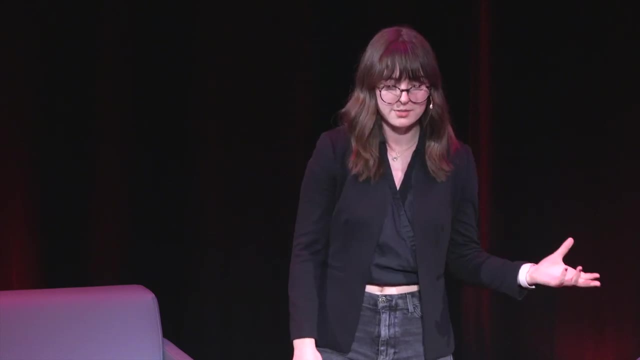 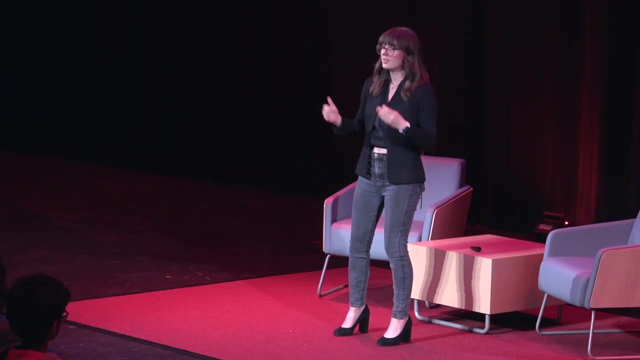 to be in a situation putting yourself in someone else's shoes. Empathy must form the backbone of our response in any issue, and especially in the issue of sexism in the STEM fields. The fourth step in the process is plan. Engineers, use this step to limit down. 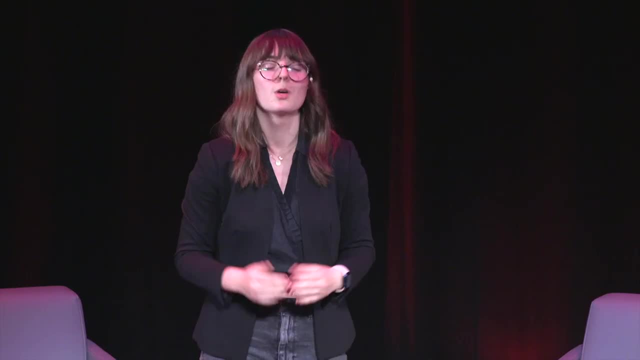 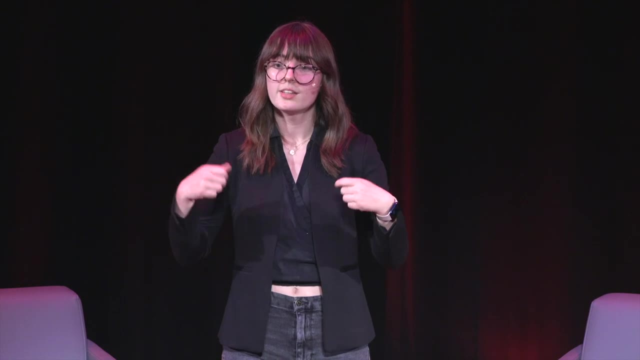 their ideas from the previous step to one or two made designs which they'll move forward with. It can be used the same way. for us, Planning is really important because now that we understand the issue, we can use it to plan for the future. We can use it to plan. 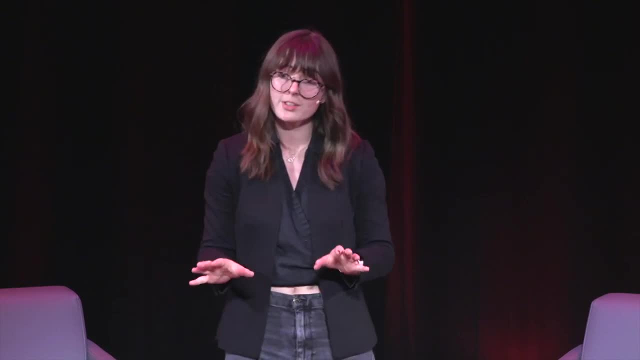 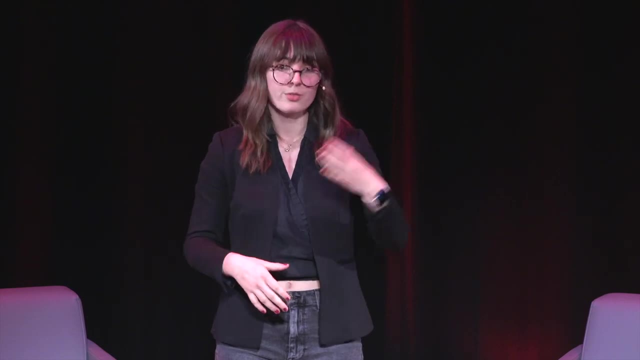 for the future. It's important not to rush forward all at once, but to carefully consider how we move forward before we do. In DarkSight, this means thinking about all of the things that we have used before and coming up with new strategies, methods and tasks to create. 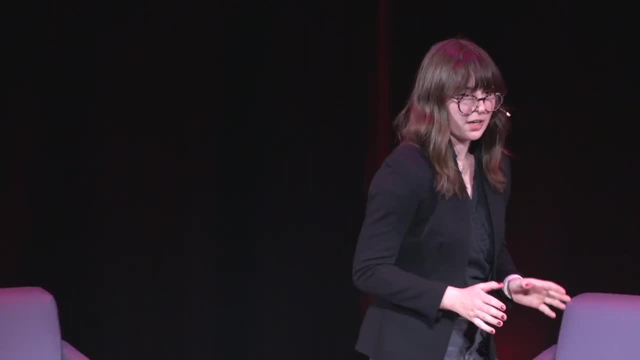 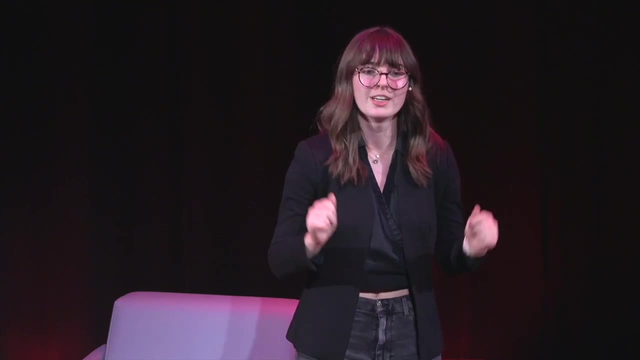 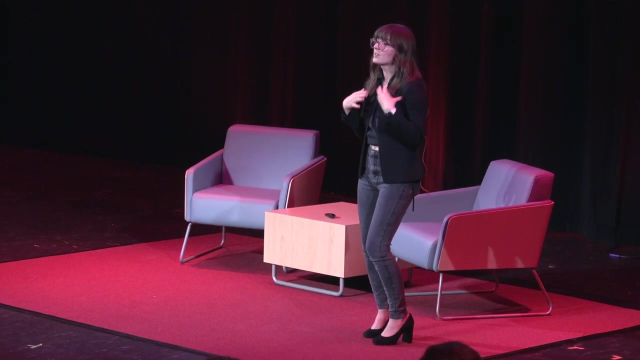 a more inclusive environment. The fifth step in the process is build and create. In a sense, we're doing the same sort of thing: building an inclusive environment. Now that we have our understanding of the problem and we have a plan of how to move forward, we must bring 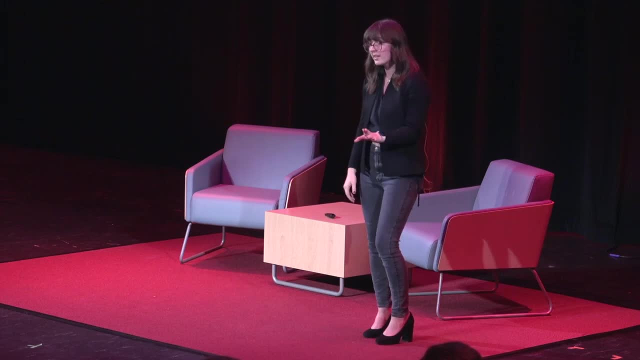 our problem solving into the real world. We must stand up for our peers, speak out against injustice and support those affected by those injustices. When combined with the sixth step- testing, ensuring what we build works and getting feedback- we arrive at the majority. 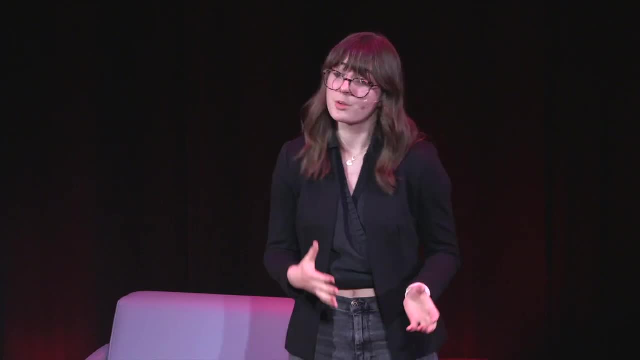 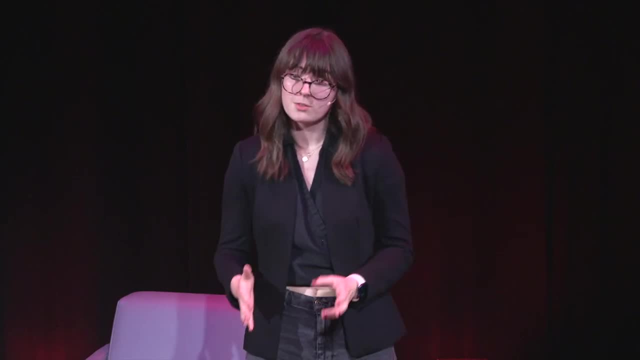 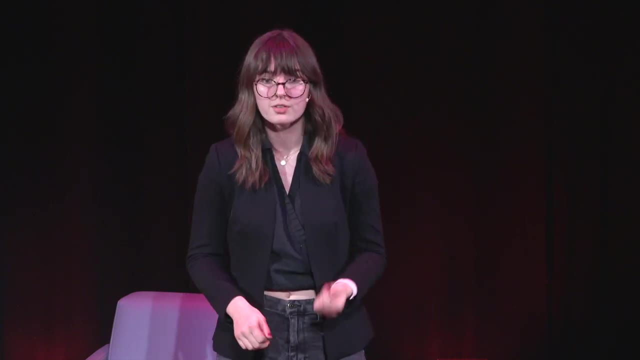 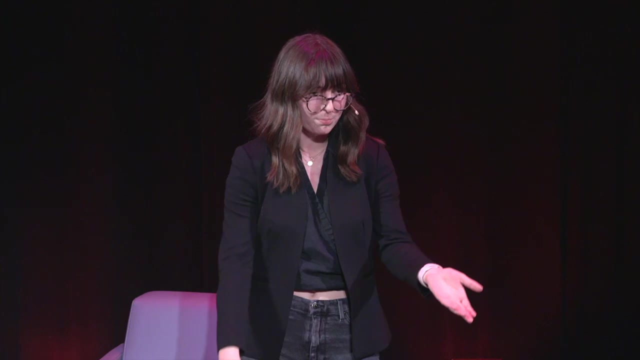 We worked to create the use of certain languages, create more inclusive spaces on the team and ensure everyone had the knowledge and support to move forward in the season. before the season started, Not everything went perfectly on the first try around. There were several things we did that we needed to correct. For example, we started having meetings at the 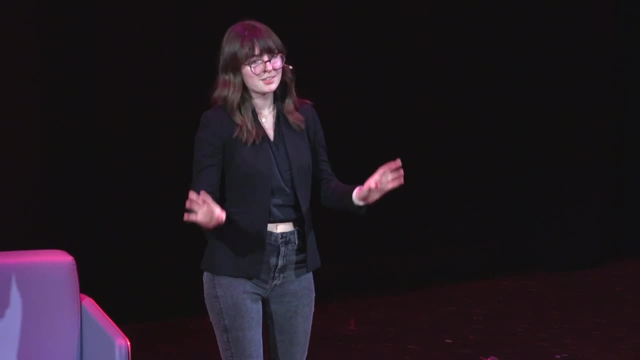 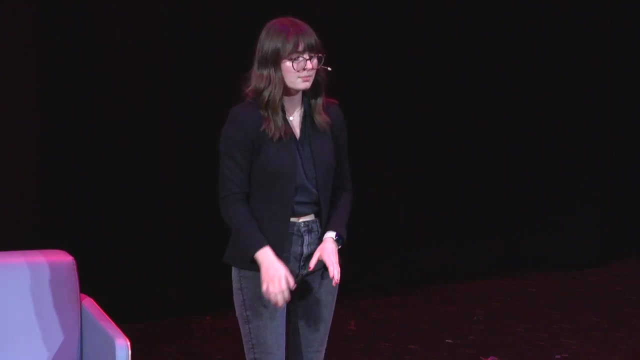 end of each practice to ensure everyone was on the same page. This didn't work because not everyone was still there by the end of practice, so we shifted those to the beginning of practices and it worked way better. Which leads us into the seventh step, the final. 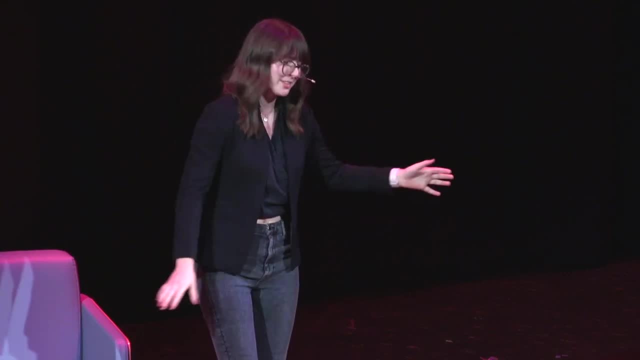 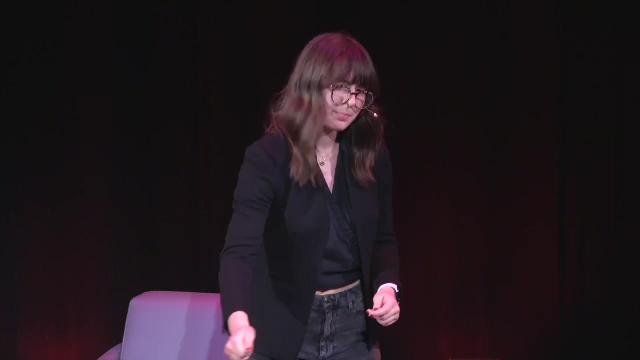 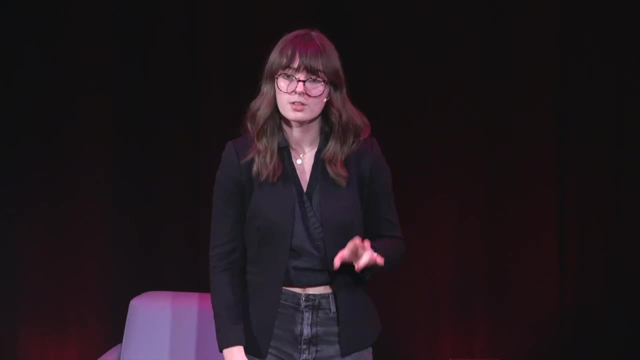 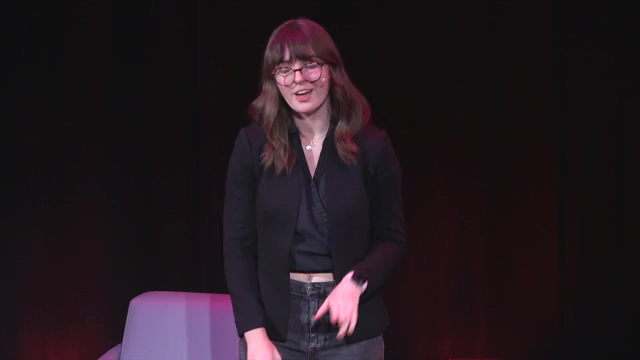 is that we're not going to be perfect. What is important, though, is that we each recognize our own mistakes and limitations and work to correct those along the way. As the season wrapped up last year, we finished a much better team than we started. I noticed us working.